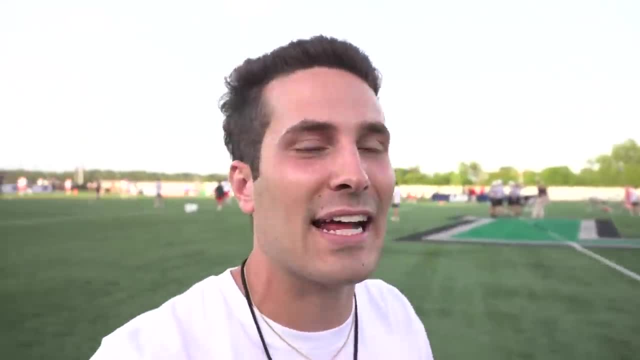 is Hilge the head coach. I don't really know. I'm kind of in between as to who exactly I want to win, but it's going to be a close game. We're out here, Coach Hill. Gardner McDonough head coach. 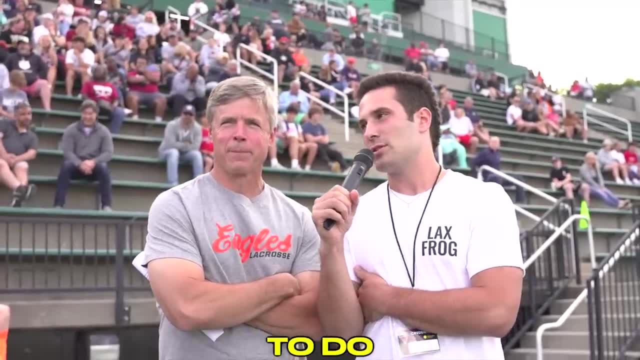 How we feeling tonight. Feeling great, Mitch, Pre-game thoughts. What do we need the McDonough boys to do in particular to get this win? Play hard, play together, play smart and stay away from you. What do you got to say to Kevin Pelkey out there? I wish we could have. 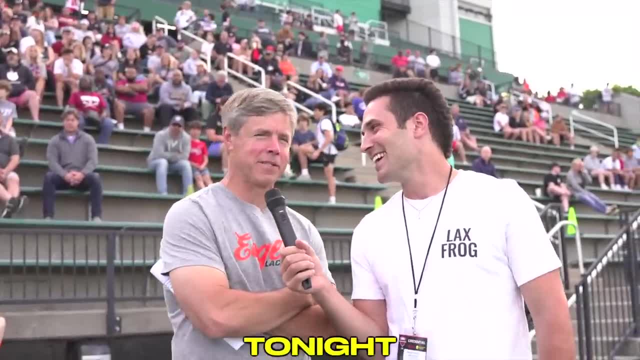 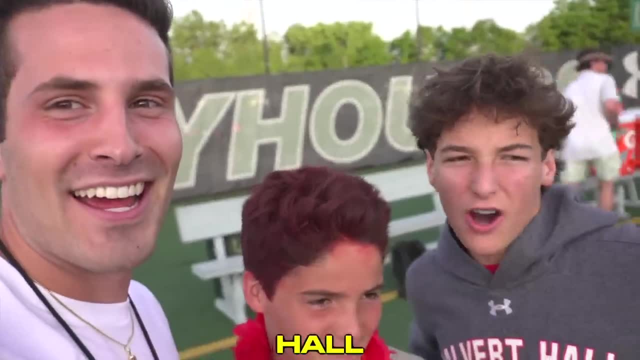 won our senior year of high school, but excited to get another chance for our McDonough boys tonight. I'm thinking McDonough 11, Calvert Hall 8.. What's the final score prediction? What do we got? 11-9 Hall, 11-9 Hall. What are we going to say to the Millen brothers? You're getting. 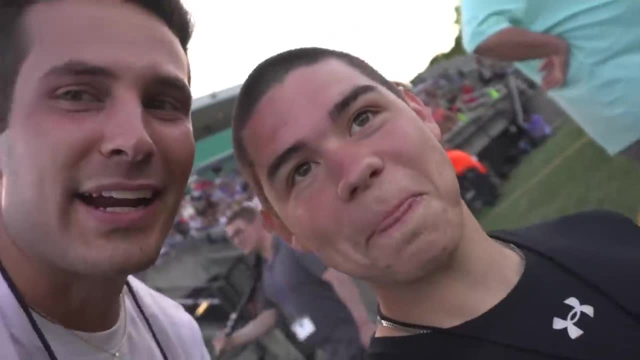 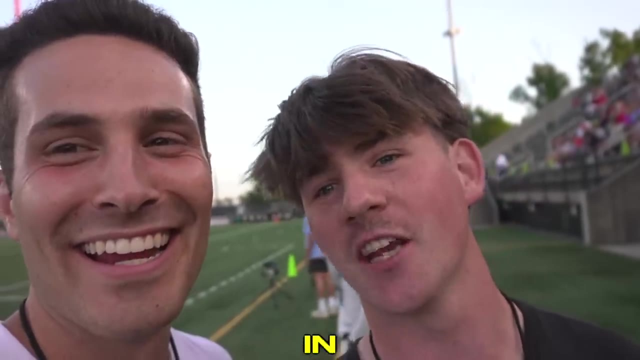 strapped McCain Actually. don't put that in. Don't put that in. Don't put that in Who we got tonight. I need a team and a score. McDonough 83-4.. I got McDonough 12-7.. McDonough: 16-15 in overtime. 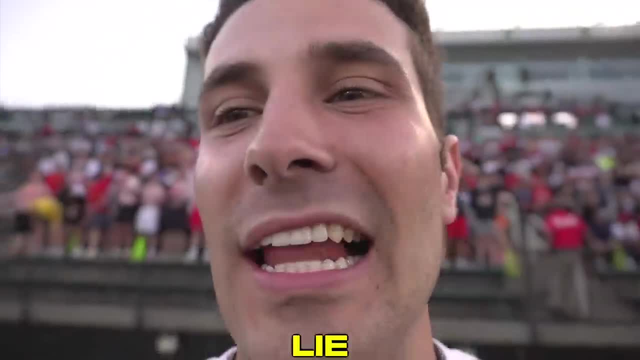 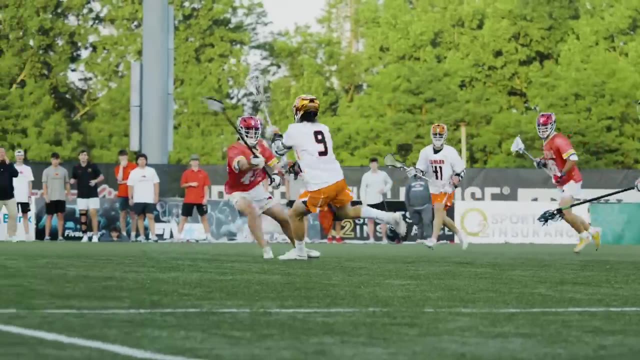 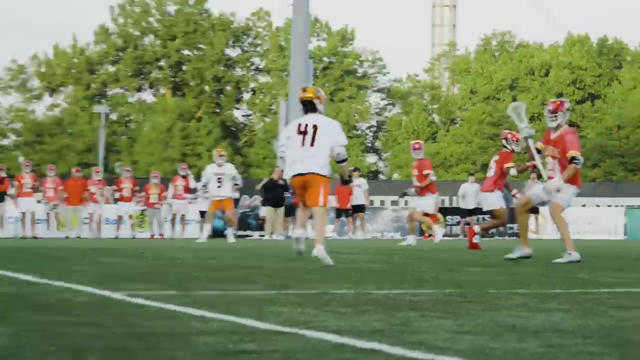 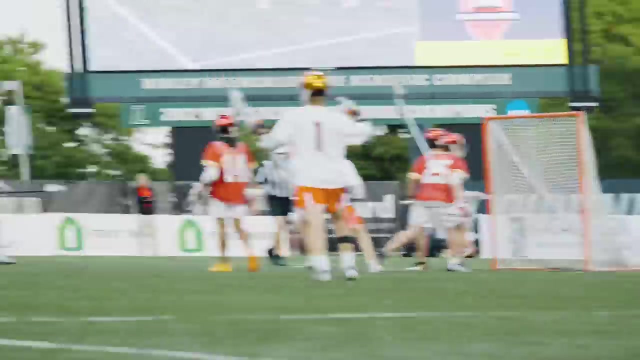 I'm not going to lie. The pre-game hype with the fans, the crowd, the music makes me miss playing. I'm not even two weeks out and I already miss it. And the shot and the score, Excellent ball movement. And three goes in. Dude, I'm telling you McDonough's going to win. 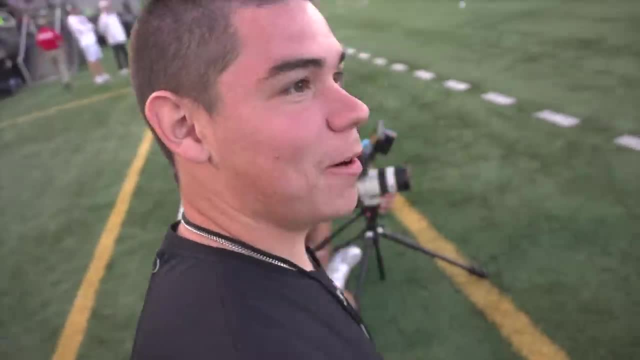 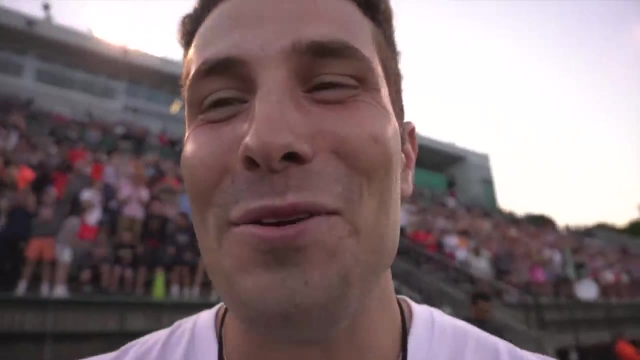 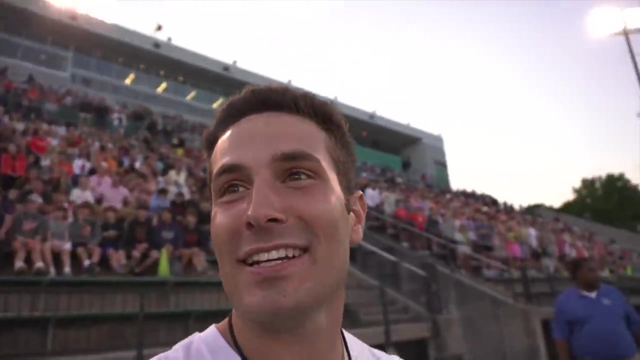 Told you 83-0.. What are your thoughts? We're on a good pace right now. Dude 41.. Millen, you're elite. All right folks, we got 10 seconds left in the first quarter. McDonough's up six. McCabe slings it. 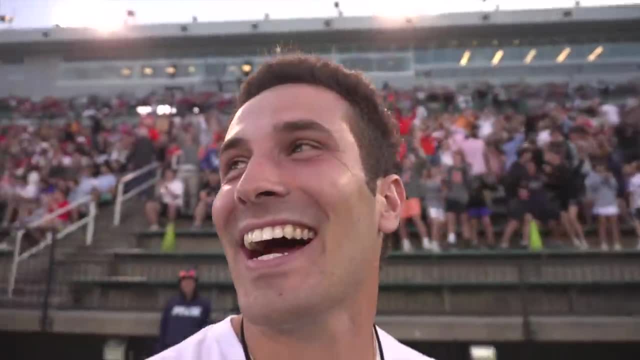 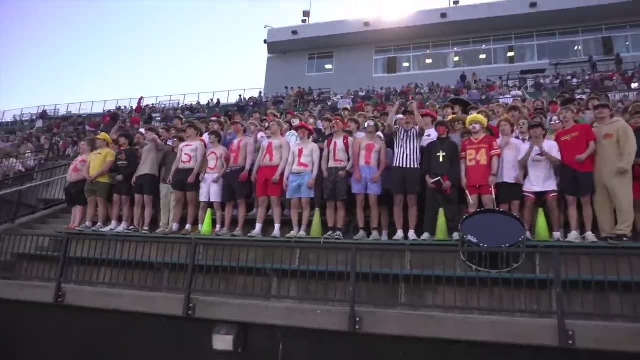 Oh my God, he's so good. Oh my God, it's 7-0.. I think Luke Miller has a hat trick in the first quarter. Mark Millen, what are you feeding the fellas? All I can say is: sexiest filmer here with that shirt on. 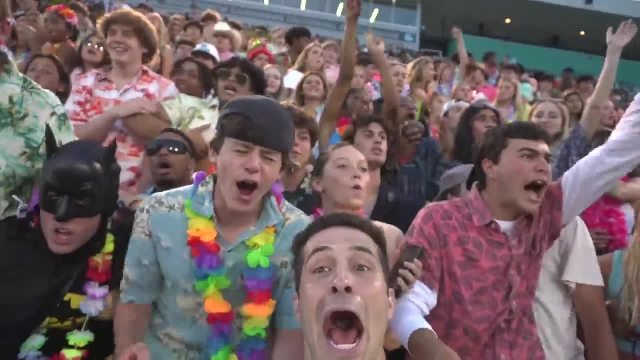 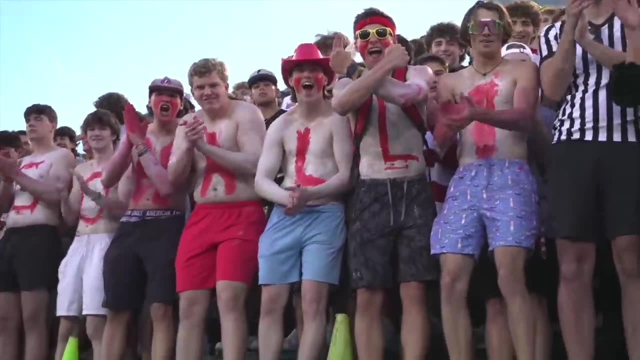 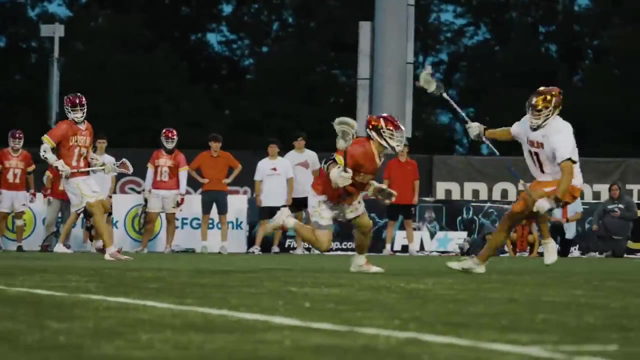 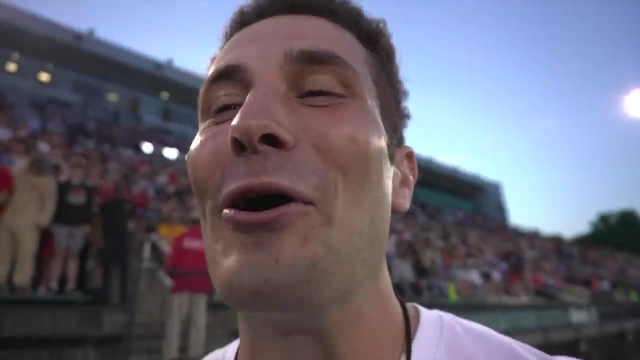 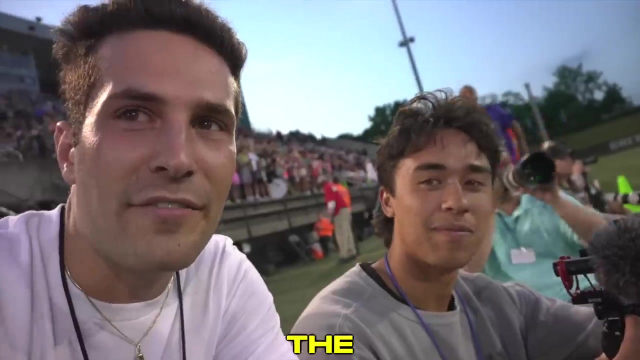 When we score, we got to go crazy. all right, 8-2.. Cavalier, two quick ones, Don't count. the haul out now. Come on, Some heinous frogs have been hit. Roll the frog reel. Tell the fans. 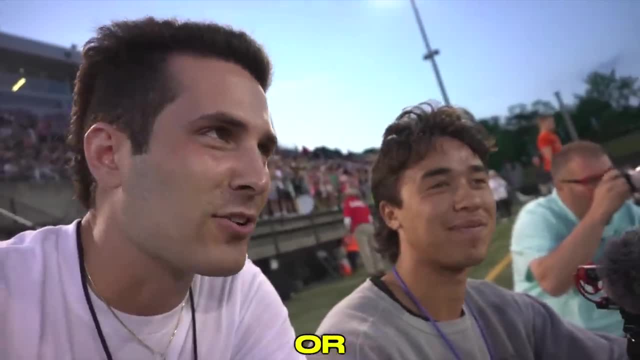 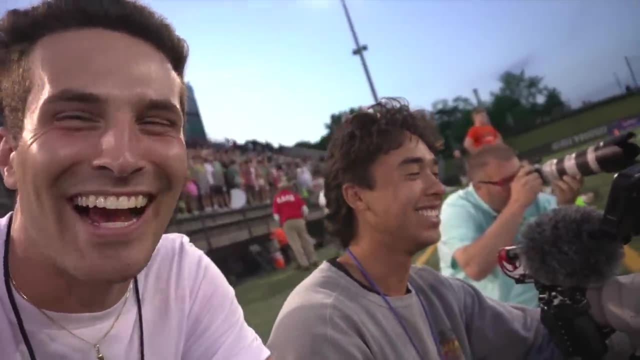 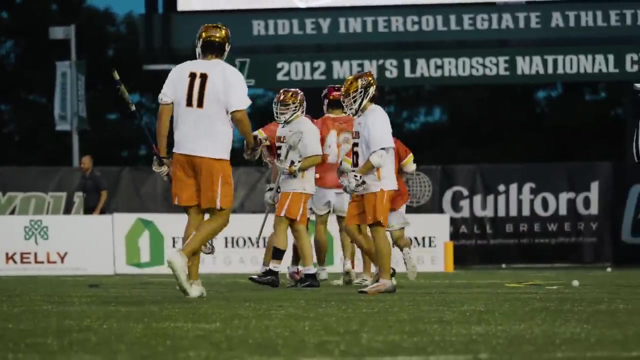 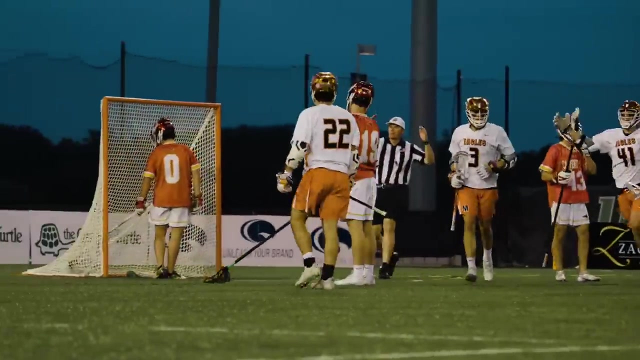 what's your Instagram? Joe K Single or taken Single. Two single Italians out here. That my championship game. Two Filipinos out here? Yeah, All right, we're here at halftime: 9-3.. McDonough's up. We're going to interview some of the fans. 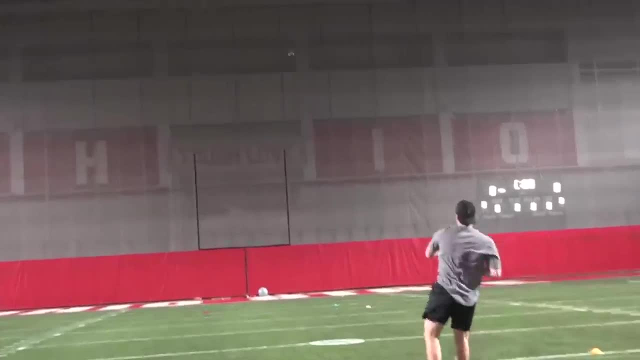 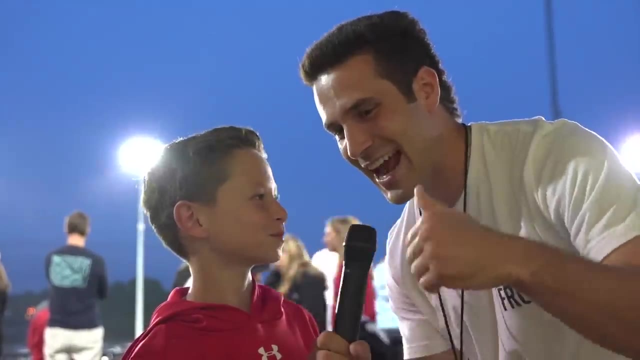 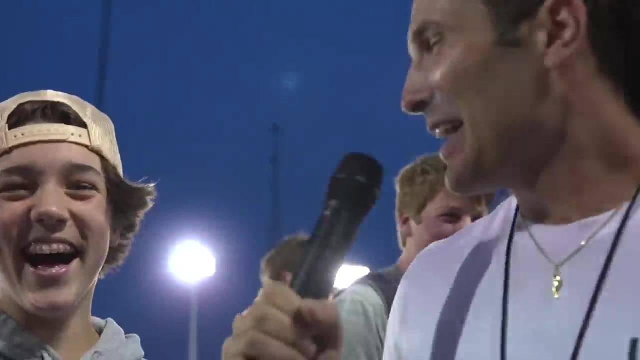 What are your thoughts about hoagie playing football? wow, hoagie's gonna play top division one football and potentially kick the national championship overtime. kick to win. yes, yeah, what's your go subscribe, subscribe, can you. can you hit the frog bing bong? this is a frog fest video. i've done a girls cross with. 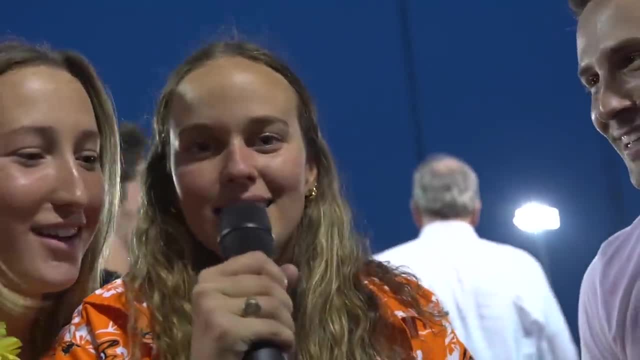 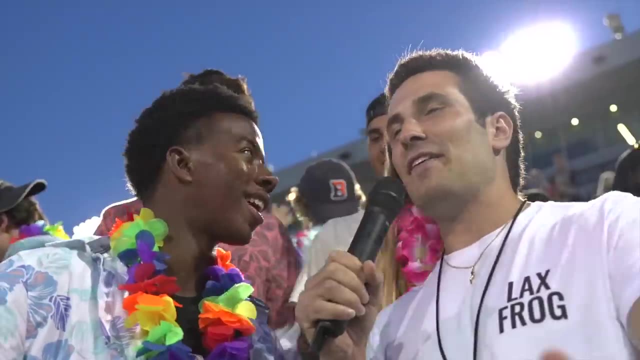 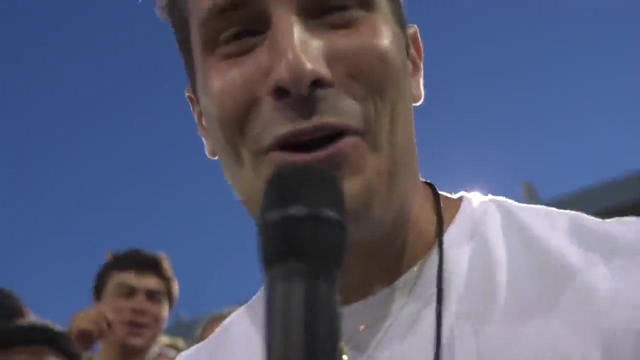 ima champions. all i gotta say is: i like my guys, mcdonough's the best. st paul sucks bing bong. merritt livermore, who is your favorite student. anna livermore, my daughter. the fans are wondering if you can hit the frog. i can hit it. let's see it. elite frogs out of the eye. what's the batman? 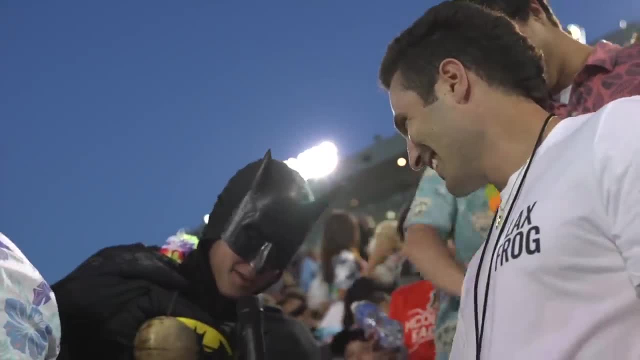 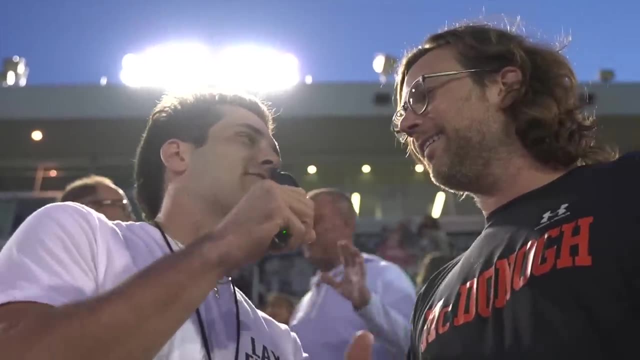 what's the batman for friday, may 19th? vengeance is here. i'll cover it all. this is uh, stephen garten 2004. mcdonough fans want to know if the class of 04 can hit the frog. bing bong, can we? 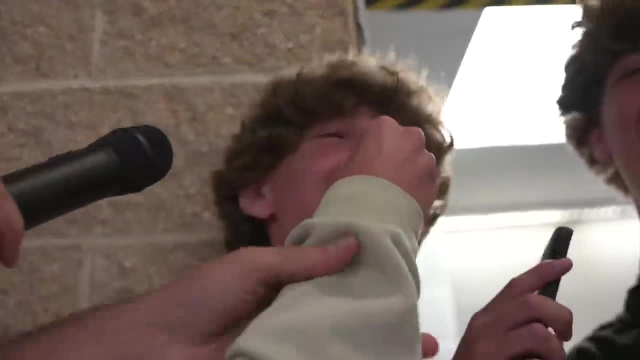 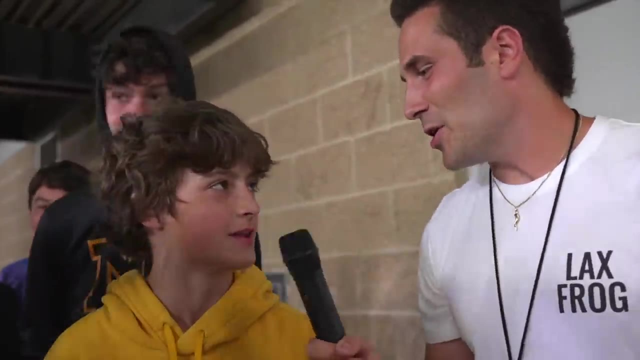 get a one bite score. this guy, deep throat glizzy from my guy, calvin mcdonough, who you got? what's the score? 21-5. emily cole. and you guys, what do you got to say to emily cole? um, you're bad, did he? heart hurts you kind of look like craig allen. who's that? 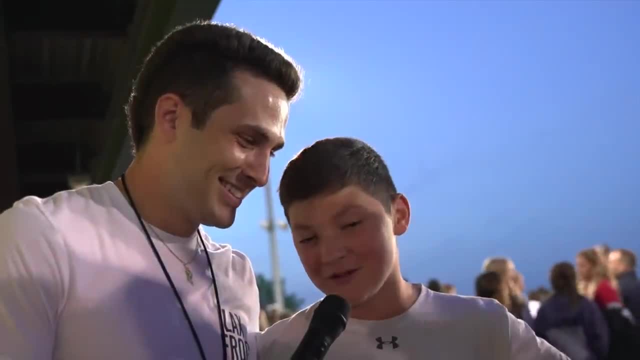 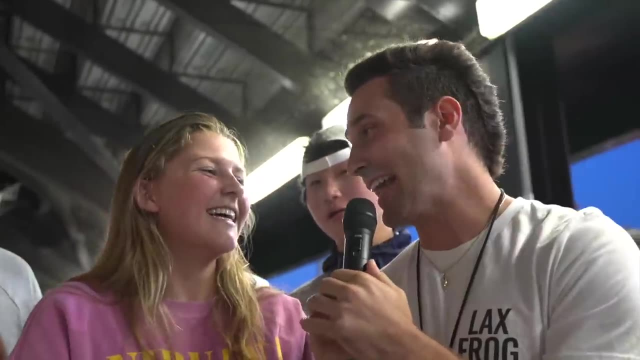 next question: what's your go-to riz line? are you a defender? because i want you sliding on me. that's what the italians do, right, ava larkin related to larkin larkin. yeah, larkin land lurking. yeah, all right, perfect size. bite larkin land, ocean city, don't forget about it. 6.8. 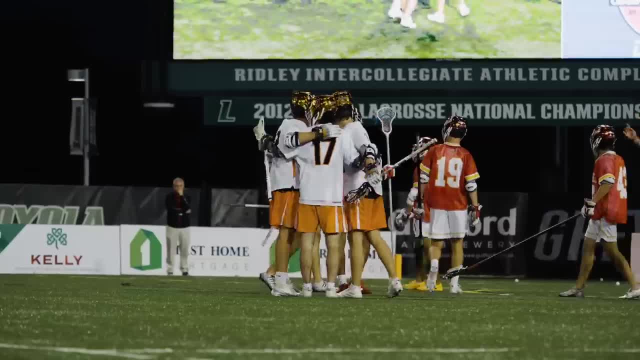 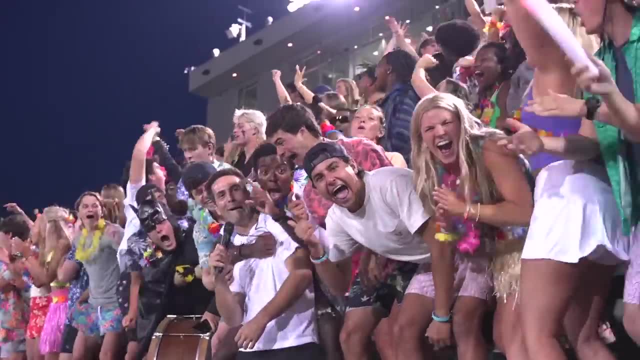 it's now 11-3. mcdonough is still up. i feel like i might need to suit up. put on kev pelkey's old jersey and hop out there for calvert hall. what do you got to say to calvin hall right now? 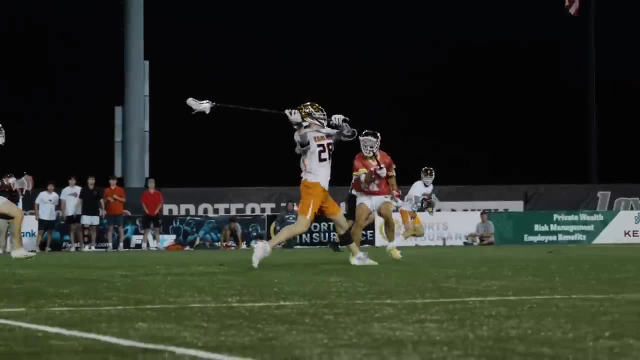 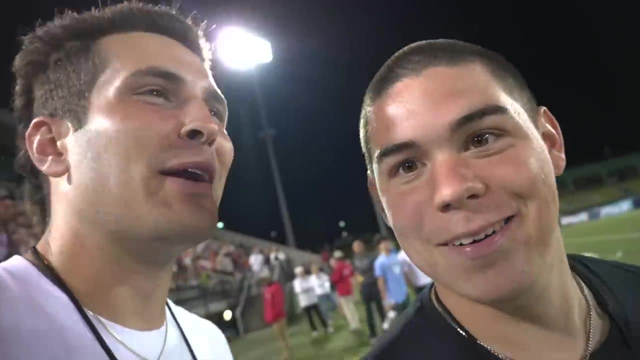 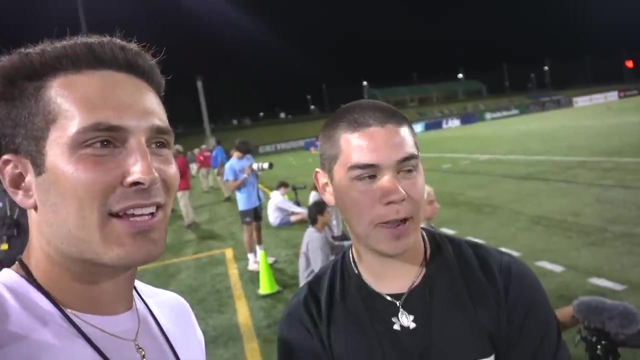 this is a clinic easel top. baby mcdonough's running away with it right now. why isn't st mary's here? tell the fans how garrett nielsen fired him up. severn rivalry game at severn down: 7-1 at halftime. boys are at an all-time low. out of nowhere we got big garrett. 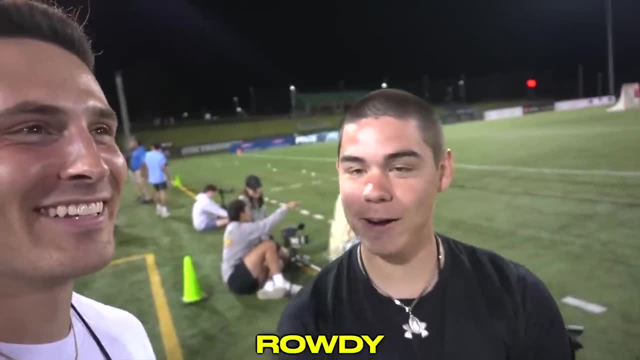 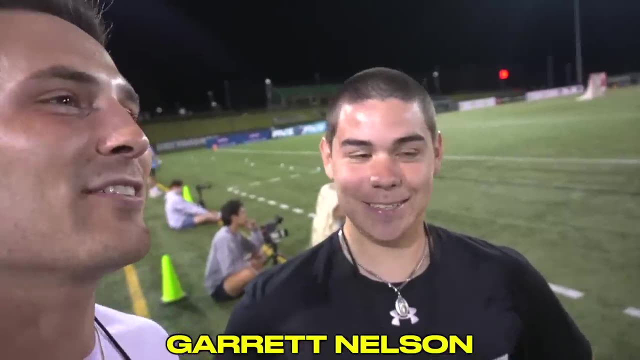 coming in to the huddle fires him up, gets the boys a little bit rowdy. slowly but surely the boys came back. boy nick galini got it done in ot celebrated all over their field. i gotta say to garrett nelson right now: all right, all right, we got five minutes left in the fourth. it's not. looking too good. the island's gonna take it home. predictions now for next year. eagles: okay, again. you think they're three peen exactly. back to back to back. how we feeling back to back, great, i mean, doing it once is amazing, but doing it twice is just. 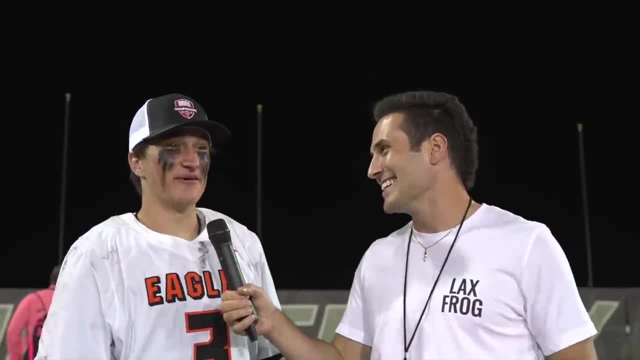 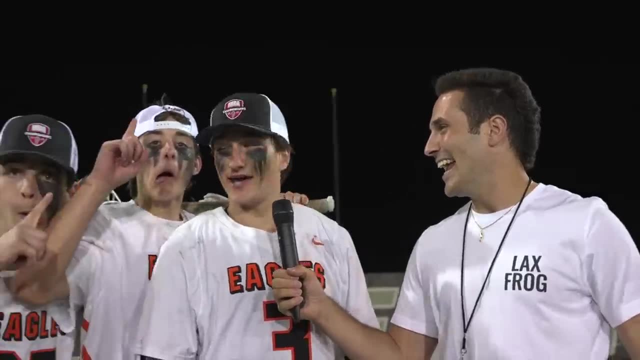 unreal people already talking about the three p. how you feeling about that? oh, definitely, but i'm definitely gonna enjoy uh tonight winning the ship. what do you gotta say to the young bucks? uh, just like, work as hard as you can, watch a lot of film, that helps the best. yeah, and hit the frog. 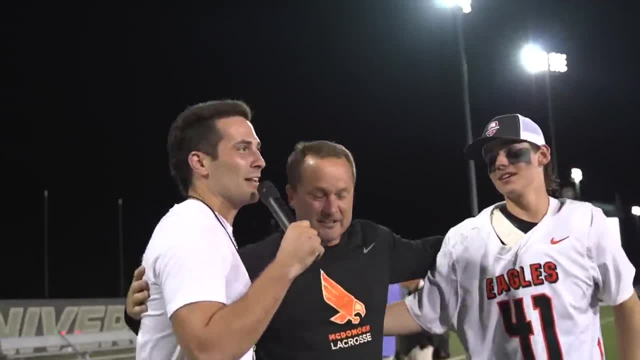 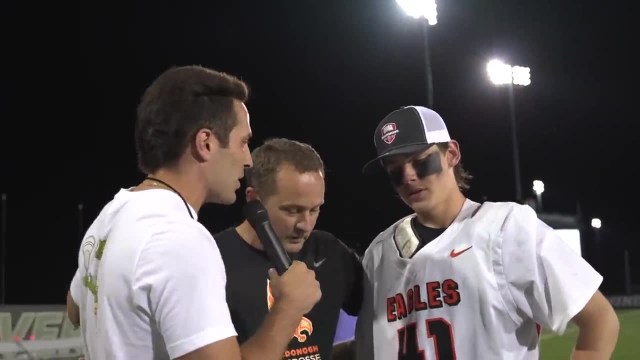 maybe, and hit the frog brendan. all right, so we're out here, mark millen, young b, how we feeling. oh my god, this is unbelievable. it's all the nights in the backyard and the bounce back in the driveway. this is what all happens, right? this is what we work for, right? you tell them asking him questions. this is the. 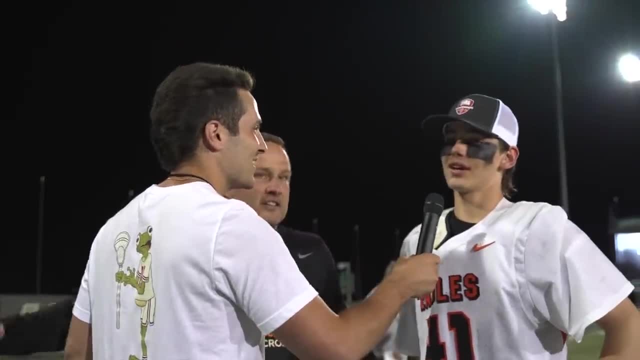 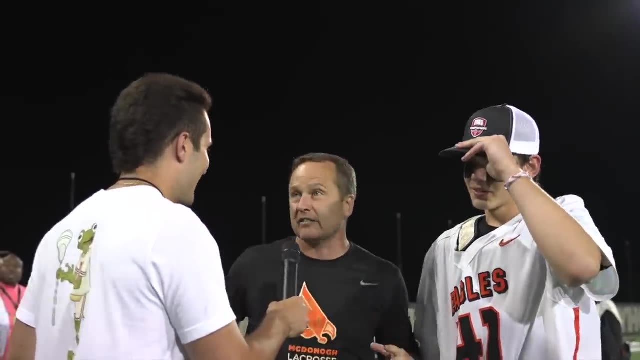 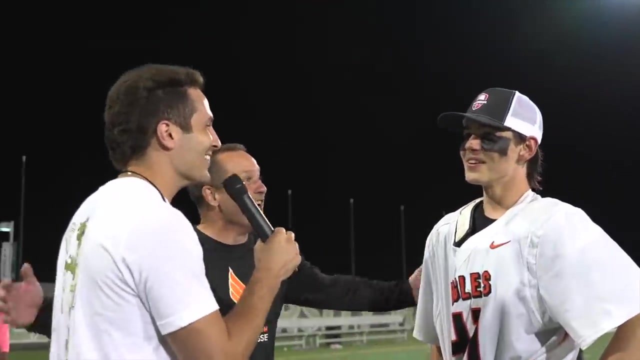 sickest thing. this is, this is what you live for. man. like to play on the stage like it's unbelievable and to do it twice. it's. it's crazy. now, when you win one championship in this league, man, it is the sickest thing. you win two in a row, oh my god, that's all i can say. i love it, i love it, i love it. a call. 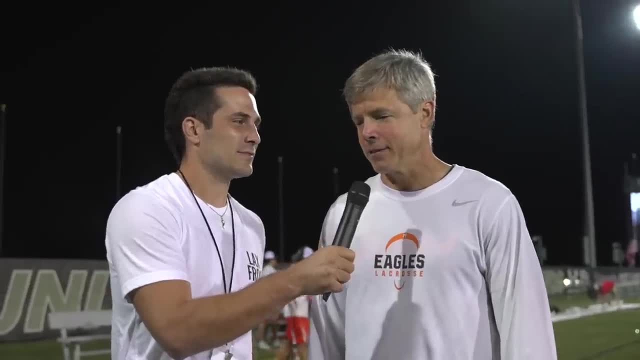 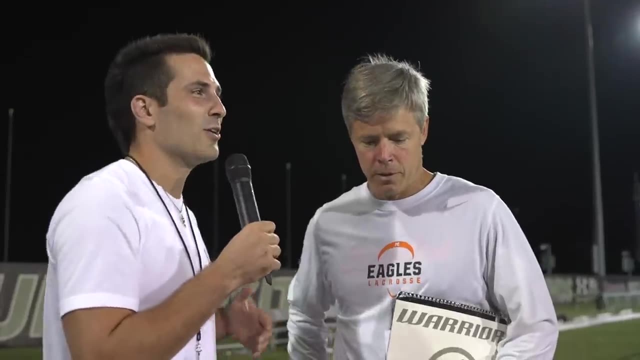 in the beginning, coach hill gardner back to back. how are we feeling? feel great man, so grateful just to be associated with the players, the coaches, everybody in our program and at our school. just feel super proud. what is coach hill guardener going to do tonight to celebrate? uh, we'll say. 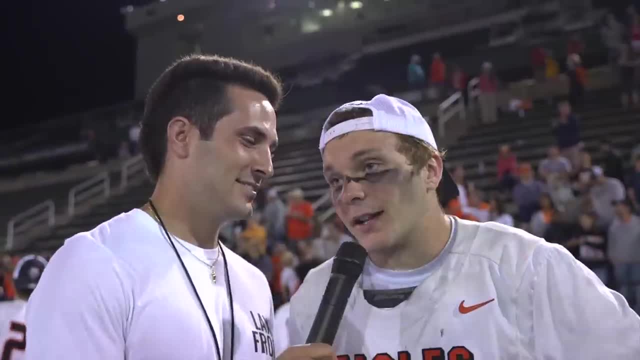 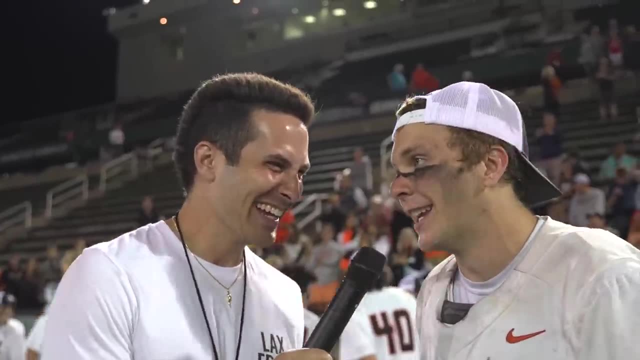 about that. all right, we got paulie the pelican air out here back to back. that is true. you kind of called it, i did call, we all called it. i'm feeling three, all feel three. no one's not feeling three. are you kidding? it's a stupid question. prediction right now: mcdonough versu next year. 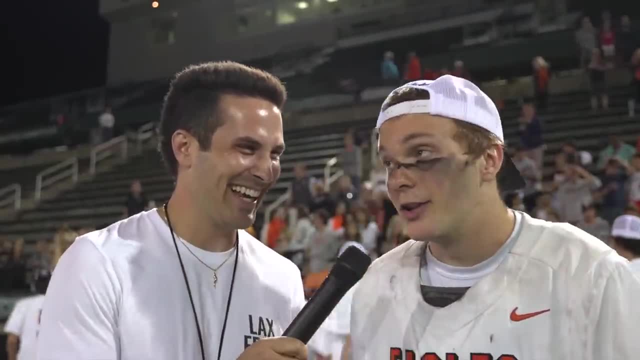 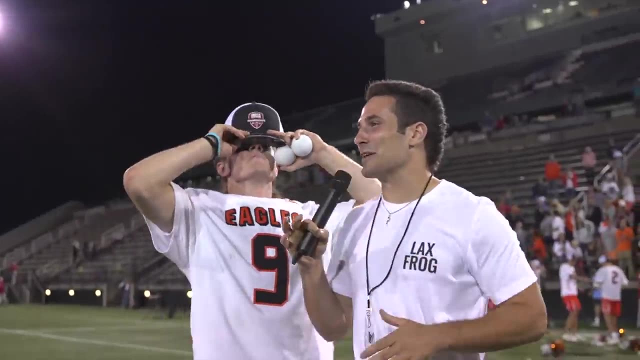 Big Dada versus the entire league. Zero goals against 200 goals for Johnny Cool's going to be at the stands, Don't forget, he's my son, Bing bong. Get up here, big boy. Last high school game ever.